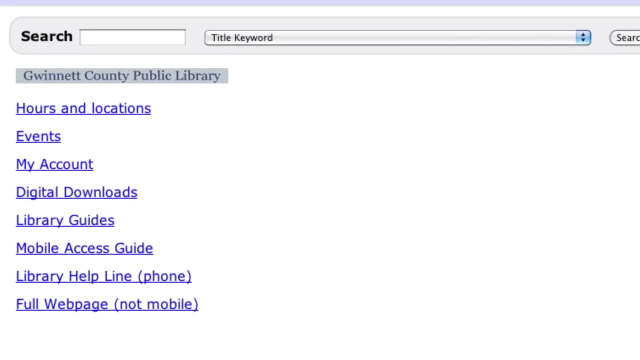 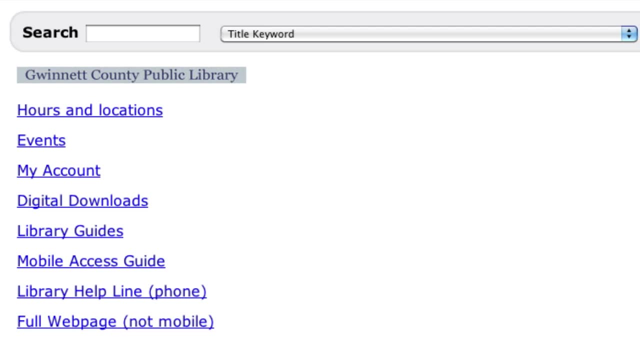 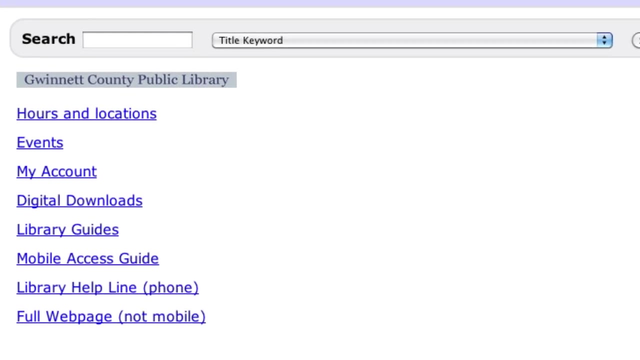 aren't as snazzy and just need the raw text. And second, it qualifies as a Section 508 accessible catalog for patrons with visual disabilities, As most OPACs today are very far from meeting accessibility guidelines. Library Anywhere is a good way to open your catalog up to all your patrons. 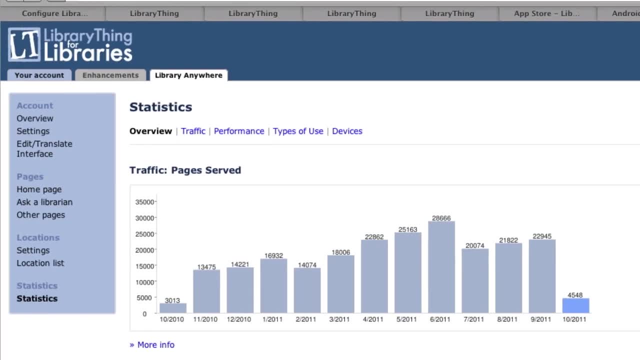 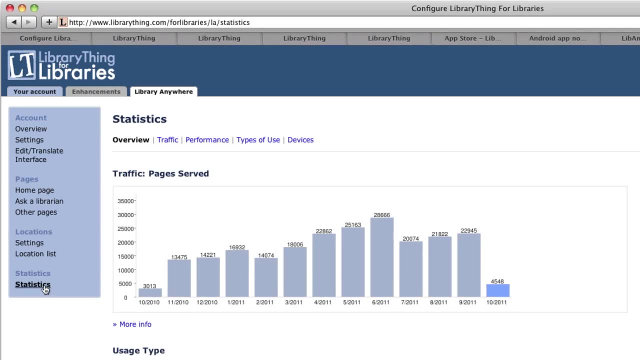 Okay, so here's the statistics page. If you you can get it by signing into your administration pages on LibraryThing for Libraries. You'll see a link down here at the bottom of statistical bottom for statistics. just click that. It's divided into five different tabs here. 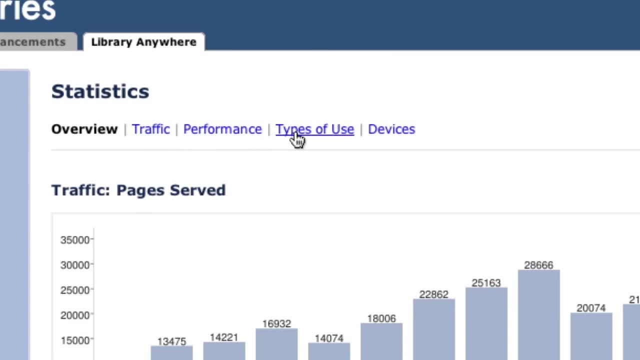 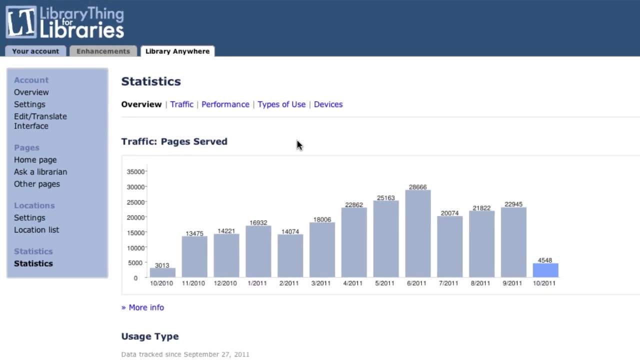 Overview: Traffic Performance, Types of Use and Devices. Now the Overview tab shows a couple of things. So we have pages served. this is how many people have been have seen looking. looking at a page on your mobile catalog, You can see it rise and fall to the current month here. 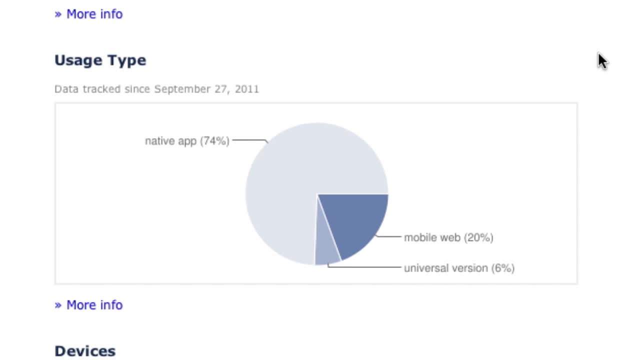 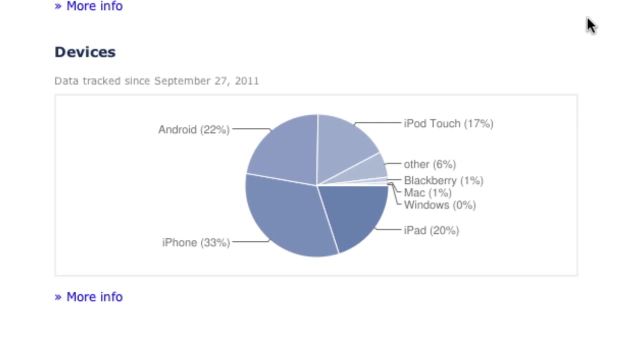 Here is usage type, So remember the three flavors I talked about. We're calling them usage type here. This is native app, mobile web and universal version. Lastly, we have devices. This shows the actual devices that people are using to access your library anywhere. 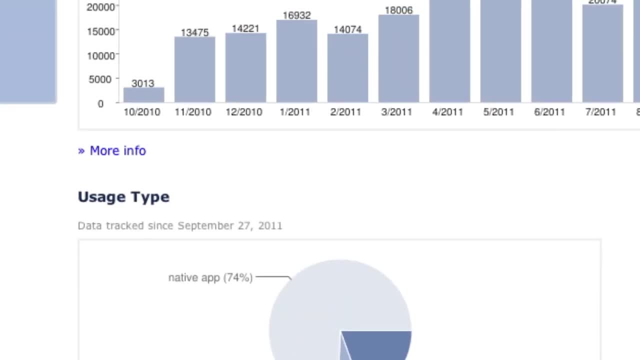 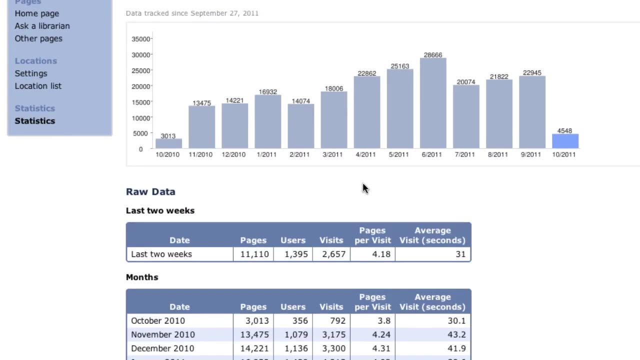 So iPhone, Android, iPad, touch and so forth. Next up, we have the traffic tab. This shows the graph you've seen before of pages that have been seen, and then raw data for the last two weeks and for every month that you've been using it. 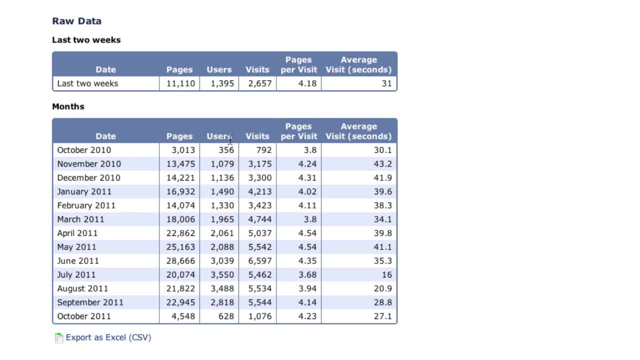 This breaks into columns like pages versus users, versus the number of visits those users did, the number of pages they looked at per visit and the length of their visits. Down here you have a link to export this data to Excel as CSV format and here you can see it. 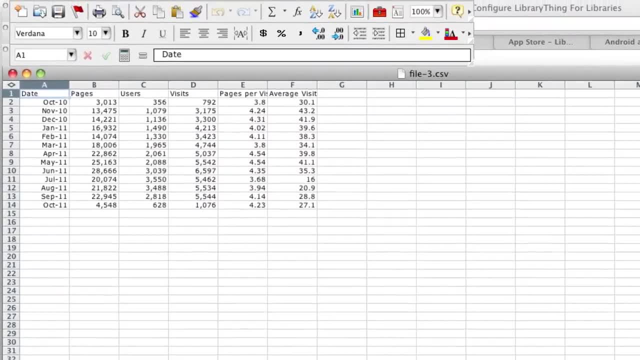 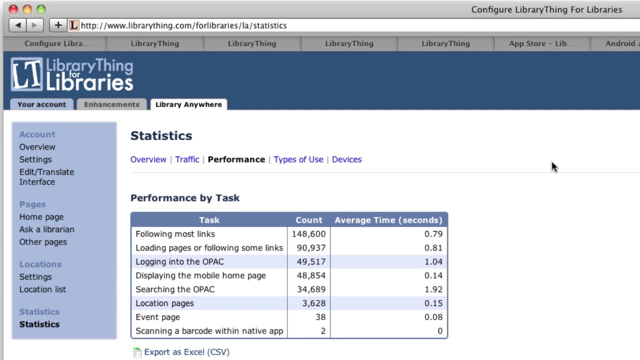 within Excel. Then we have the performance tab. The performance tab shows you a number of the common tasks and how long they took For most libraries. you'll be interested in how many searches people did and how fast they were and how many times they looked at your mobile homepage. 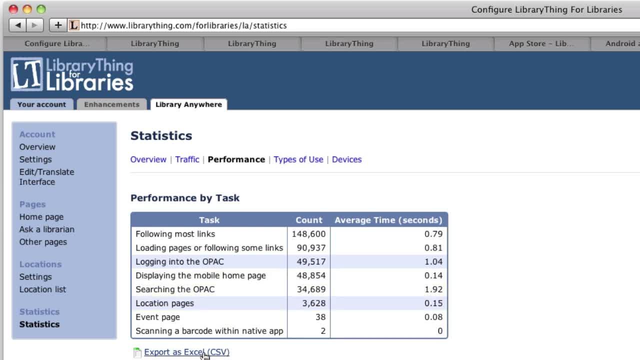 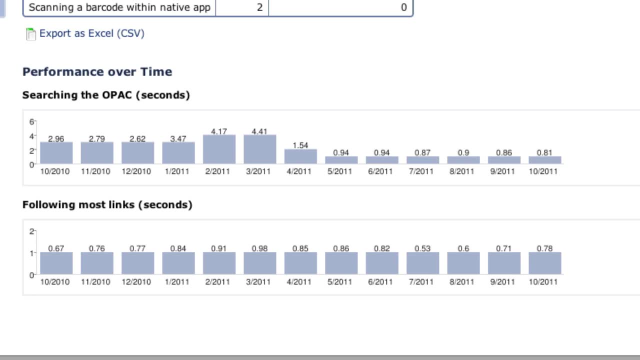 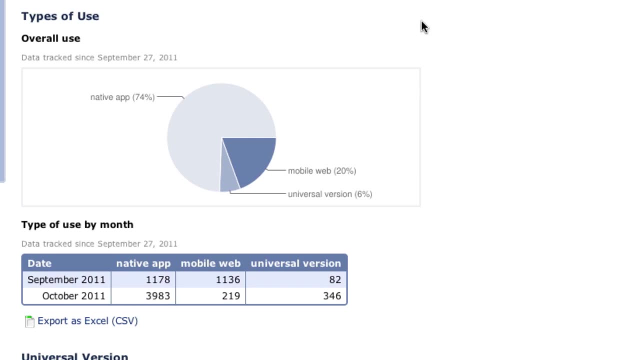 You can also click to get an Excel version of that. here You can also see performance over time. This library here did something to their search and now it's faster. Here is types of use. So here are these three flavors again: native app, mobile web and universal version.